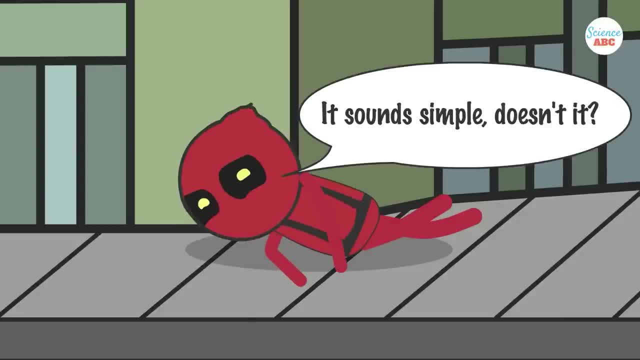 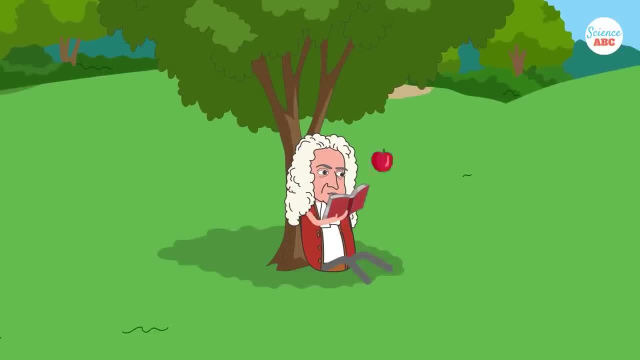 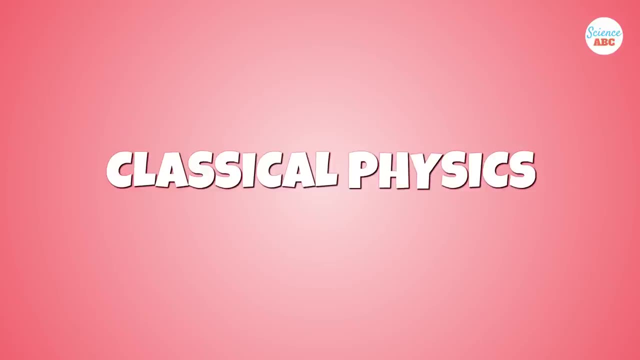 both matter and energy. That sounds pretty simple, right? So how is this any different from regular physics? The regular physics is the physics that deal with Newton's laws of motion and its related mechanics. This is more formally called classical physics. This is the physics of our day to day lives: the rolling of balls. 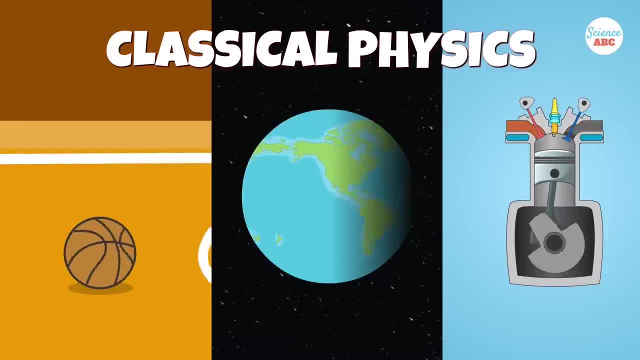 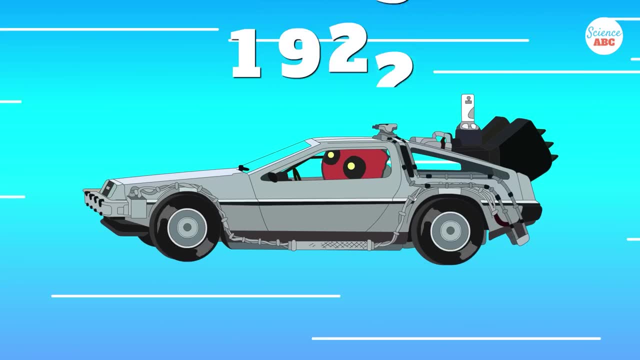 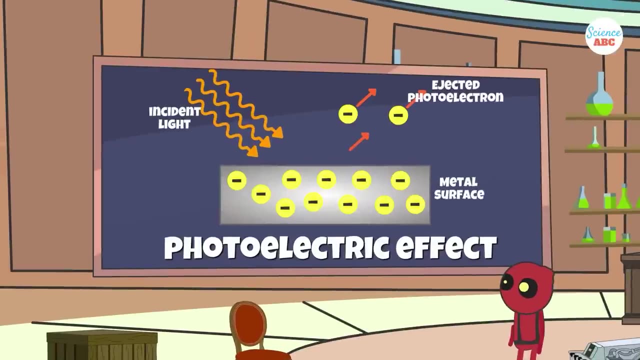 the rotation of the earth and the mechanics of engines. However, if classical physics is so wide-ranging, why was it insufficient? We must go back in time to the 1900s to witness the birth of quantum physics. This was a time when scientists were still unable to understand the observations of the 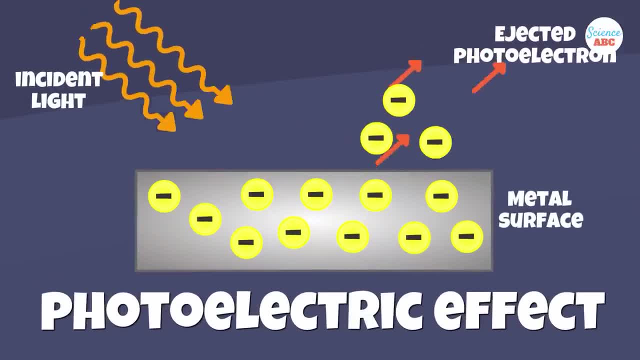 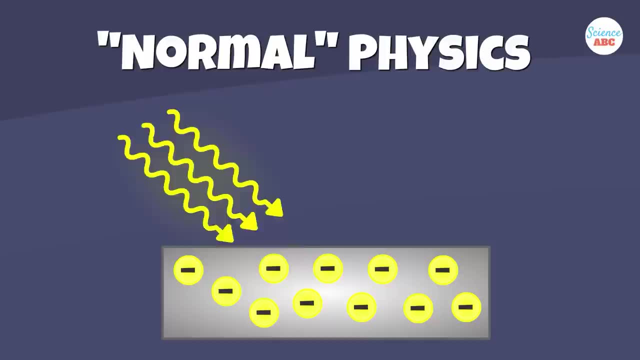 photoelectric effect. Simply put, the photoelectric effect is a phenomenon in which light hits metal, resulting in the knocking off of electrical energy. According to normal physics, the electrons should start escaping the metal when the brightness of the light exceeds a sufficient limit. 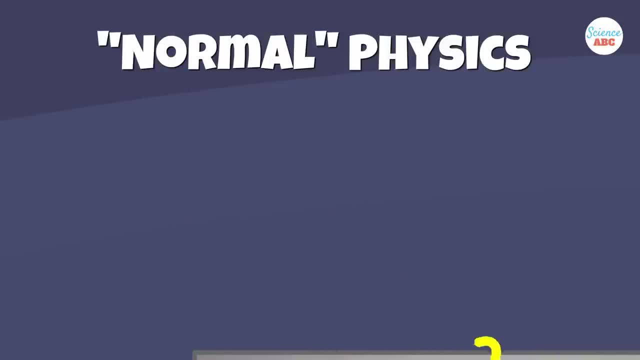 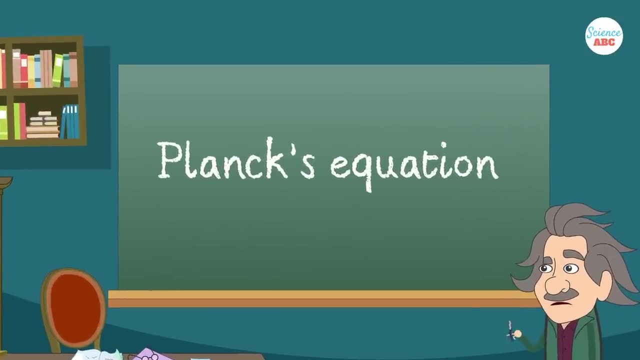 Yet in reality, it was the color of light that determined whether electrons would be emitted or not. This was when Albert Einstein turned to Max Planck's equation. Planck's equation stated that light waves carry energy in small packets called quanta. 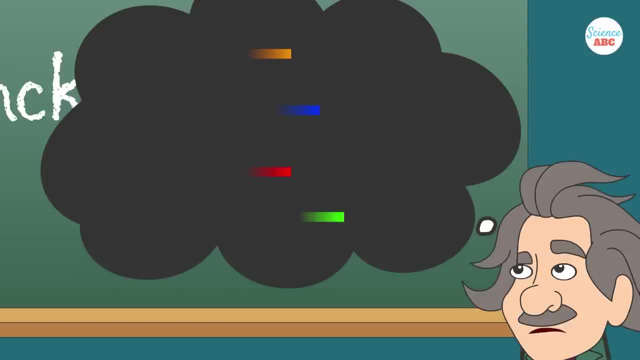 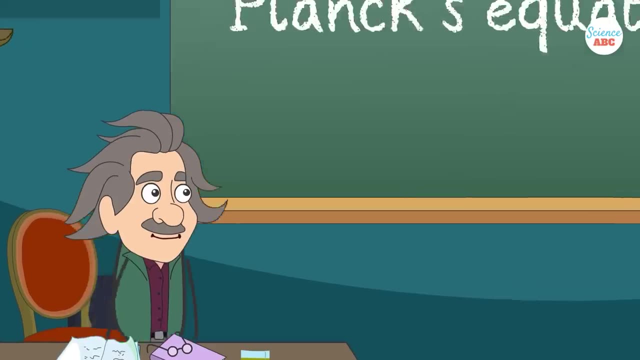 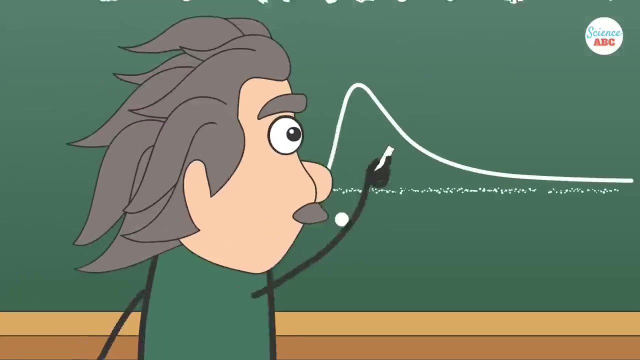 This explained how each color of light had a specific amount of energy associated with its wavelength. This energy in turn was responsible for the electrons getting knocked off. Einstein used Planck's equation to propose that light not only acts as a wave, but also as a particle, a particle later named photon. 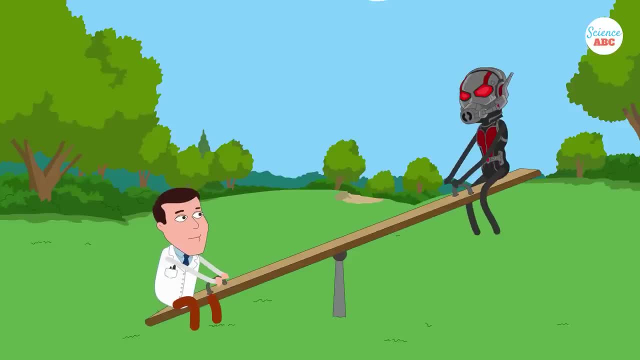 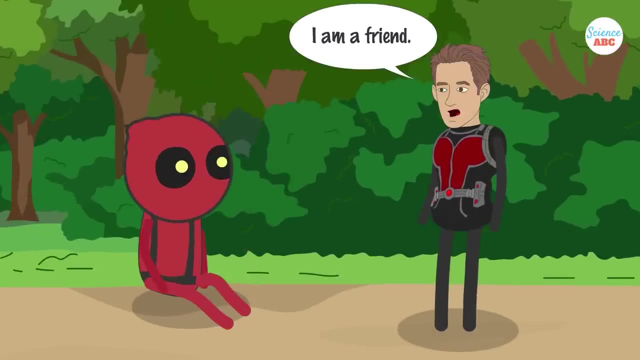 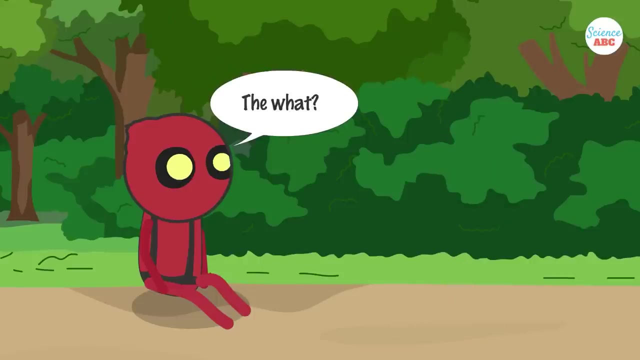 Since then, physicists realized that regular physics simply wasn't sufficient to understand the microscopic world. They termed this regular physics classical physics, a physics of the past, and another branch of physics dealing with the fundamental world, as quantum physics. This world is therefore now called the quantum world. 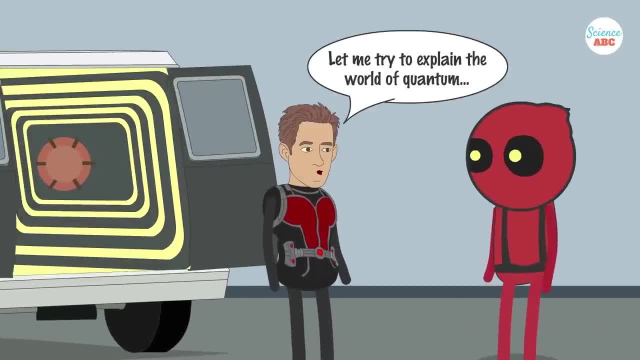 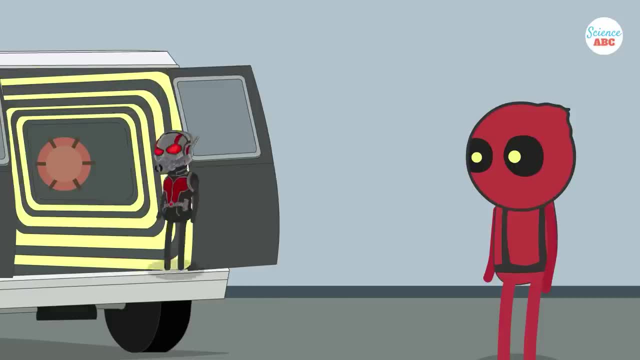 Let's be honest. our brains are made for this macroscopic world, where they can understand the running of a car on a road or the mechanics of a pen, But they are unable to initially understand the quantum world. For instance, imagine you're standing in front of a massive wall and want to reach the other side. 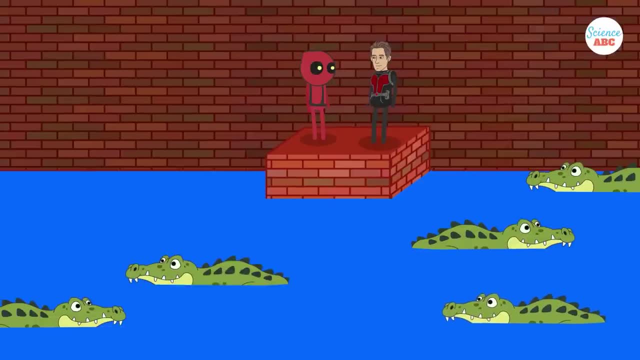 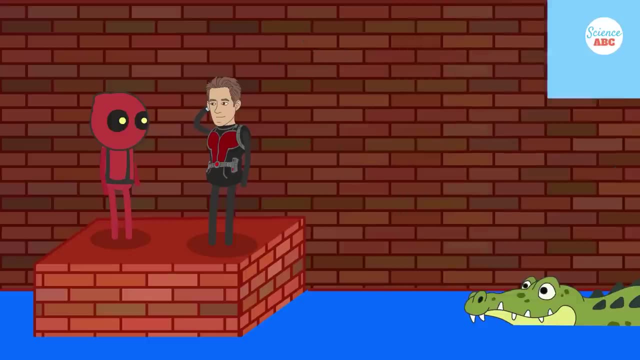 This wall is surrounded by deadly alligators, so your only options are either climbing it or making a hole through it. However, if you don't have energy, you can't climb it. If you don't have energy enough to do either, you won't be able to reach the other side right. 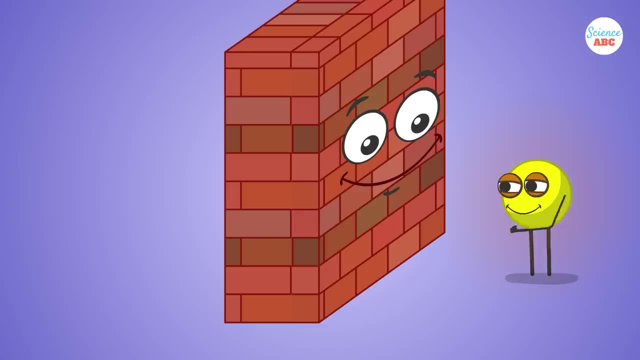 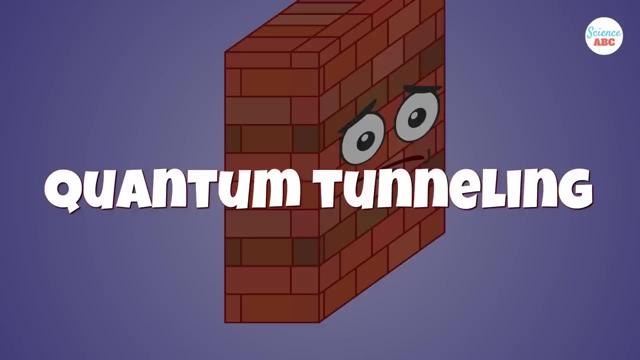 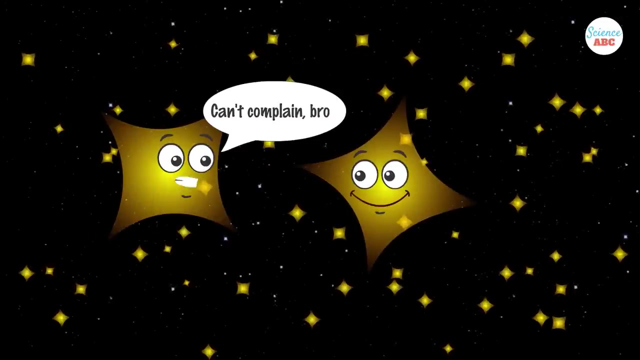 Well, that's how the macroscopic world works, But in the quantum world, a particle can still go through such an energy barrier without sufficient energy. This ability is called quantum tunneling. This phenomenon is responsible for the nuclear fusion that fuels the energy production of stars. 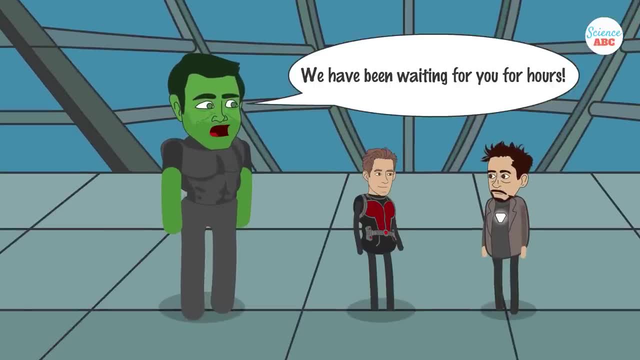 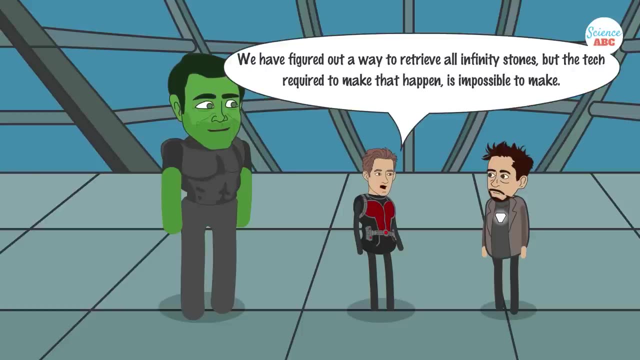 As complicated as quantum mechanics may seem to some, it gets special love from popular culture. You may often see the dramatization. It's the manifestation of unusual quantum phenomena depicted in our macroscopic world through movies and TV shows. Take, for instance, the Marvel universe. 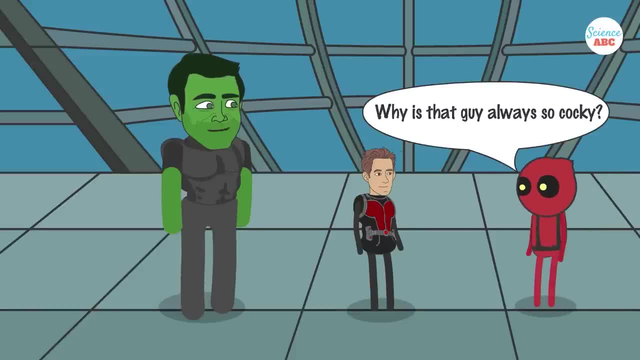 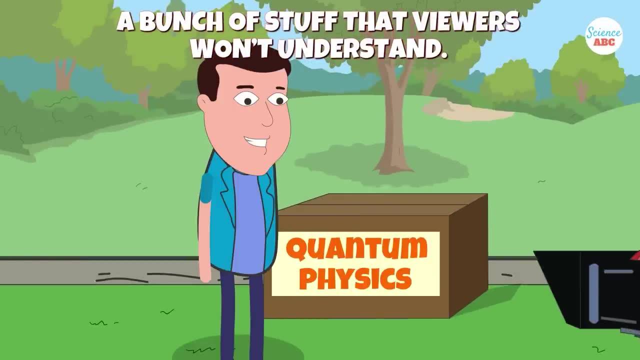 Marvel movies are famous for their heavy use of quantum physics- at least the words, if not the actual physics. Even though most of it is fiction being labeled as quantum physics, there are some scenes that are based on theoretical concepts. One of these is the multiple realities of Doctor Strange. 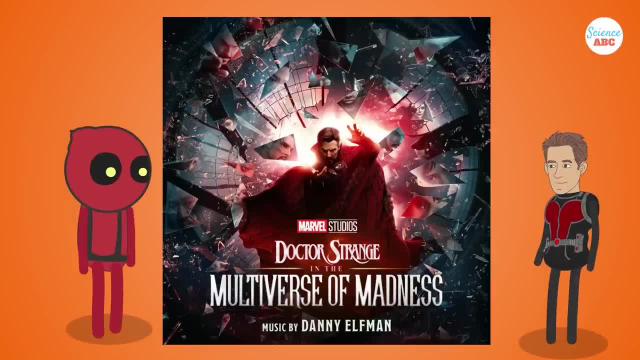 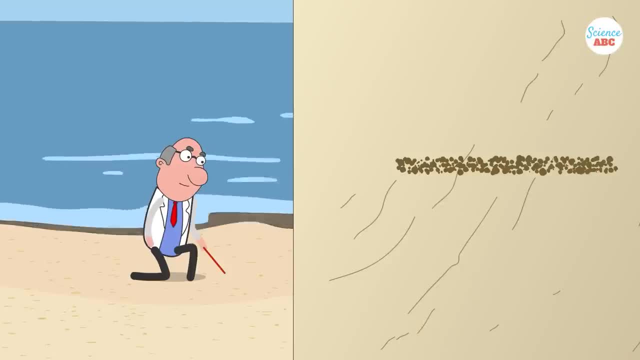 First let's understand the quantum physics on which it is based. This subject deals with particles in terms of probabilities. For instance, while talking about the position of an electron, a physicist might say the electron is most likely to exist in this range of lengths, say, between one to three units. 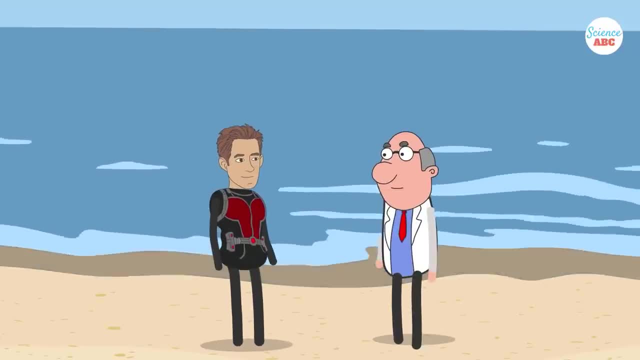 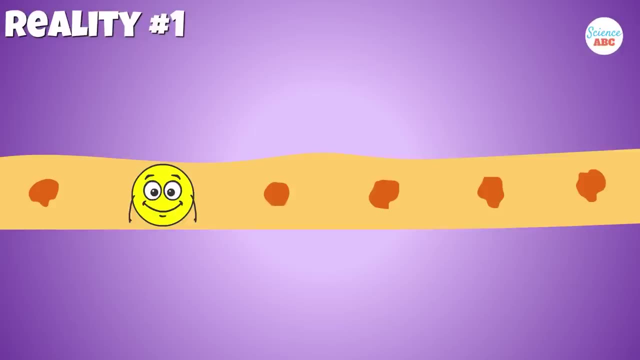 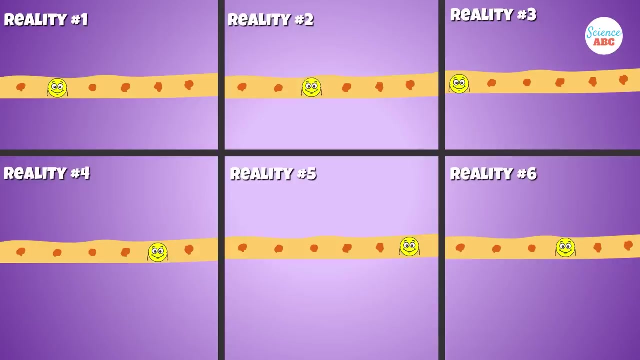 However, the same thing can be interpreted as electrons existing in different realities at different positions in the possible range, So it can exist at two units in one reality while at three in another reality or any other possible number between its possible range. In short, there are many realities covering each possible position of the particle. 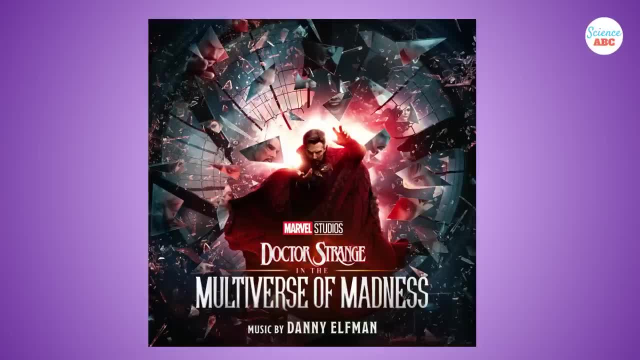 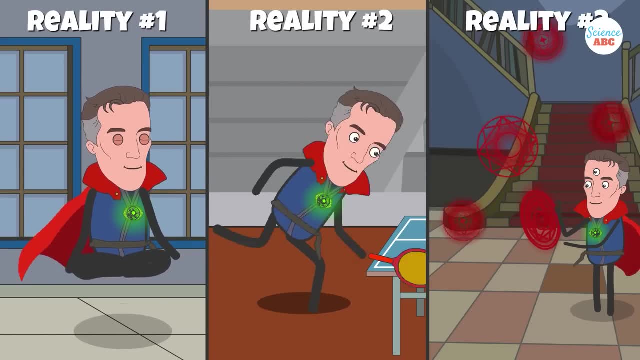 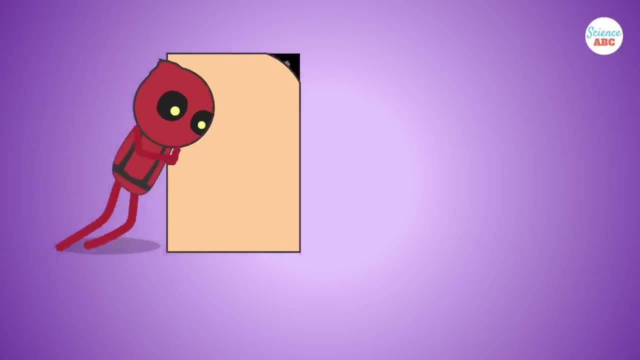 See mathematics and its implications again. A massive magnification of this concept is what we see in Doctor Strange's Multiple Realities: Each possibility of a reality is a separate universe in itself, allowing there to be multiple universes. Another very famous use of this concept is in the beloved movie Endgame, specifically its idea of time travel. 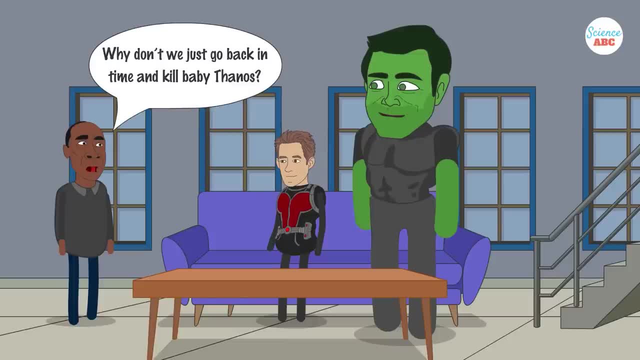 The movie understands the logic of time travel. stands that if we change the past, the future will also be changed. So if they all go back in time and kill Thanos, who will bring about the apocalypse? and why would someone travel back in?